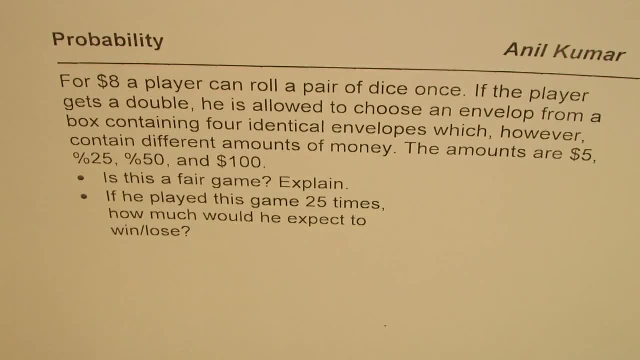 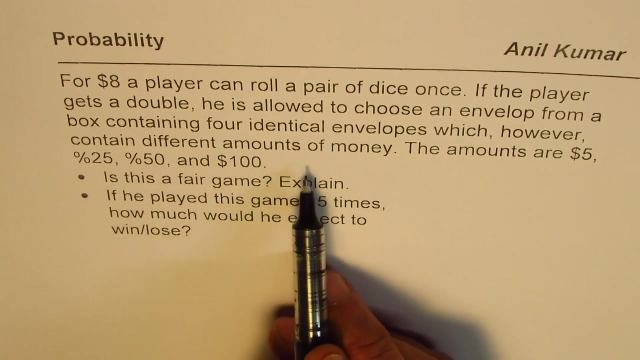 I am Anil Kumar, sharing with you questions from my student's assignment. The question here is: for $1.08, a player can roll a pair of dice once. If the player gets a double, he is allowed to choose an envelope from a box containing four identical envelopes which, however, contain different amounts of money. 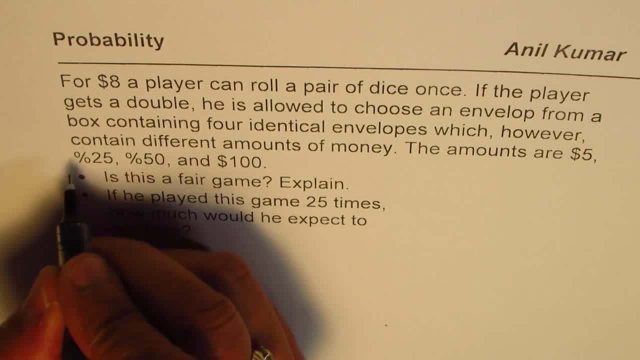 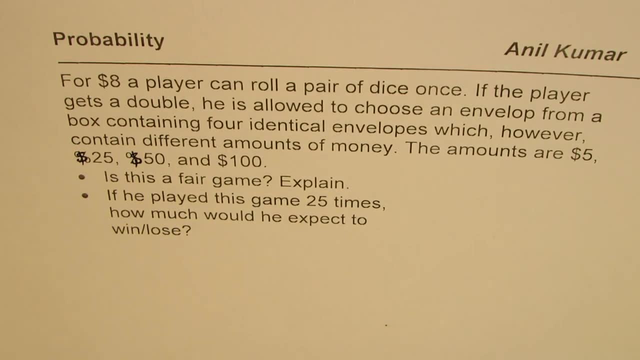 The amounts are $1.05,, $1.25,, $1.50, and $100.. Now you have two questions based on this information. Is this a fair game? Explain: If he played this game 25 times, how much would he expect to win or lose? So that's the question for you. You can pause the video, answer the question and then look into my suggestions. 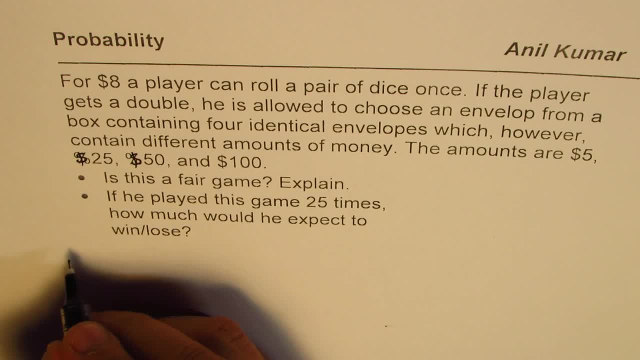 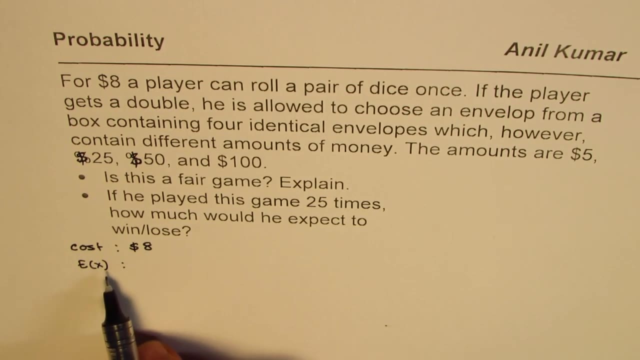 Now, let's remember, the cost of the game is $8, right? So win or lose really depends on what is the expected value. If the expected value is $8, then it's neither, But if it's less than $8, you're losing that money. If you gain, this expected value should be higher, right? So that's the concept. 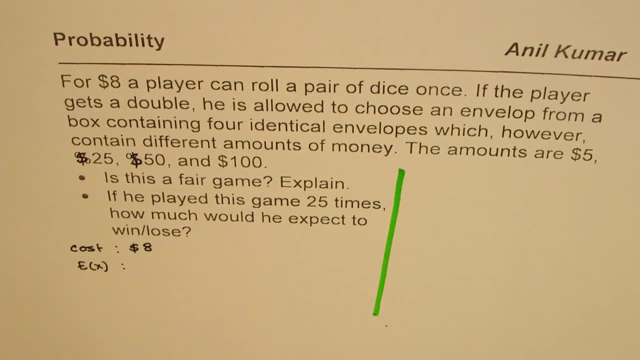 Now you can always answer the question. Here is a share, Here is a shortcut solution to this. We are saying: is this game a fair game or not? So now, the first thing is: when you roll a pair of dice, what is the probability of getting a double? Now, when we say double, it means what? 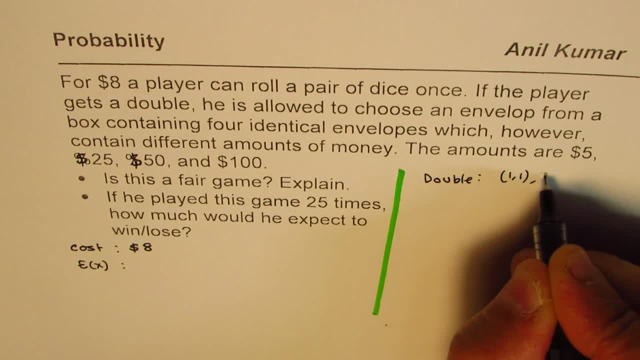 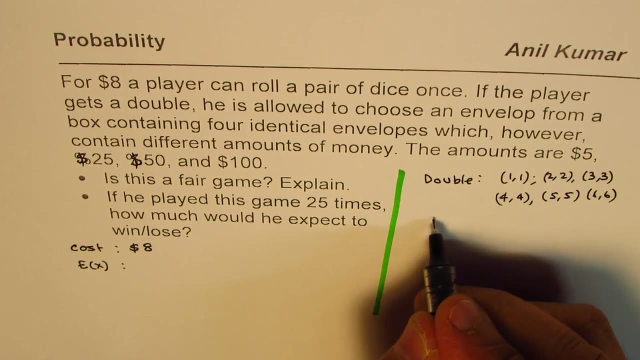 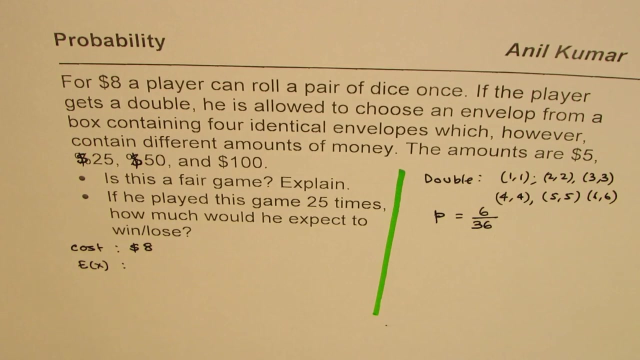 Double means you get 1-1, or you get 2-2, or you could get 3-3,, 4-4.. So both dice have Have the same value. Then you have a double right. So that is possible. So the probability for this success is 6 out of 36, right, These are the six combinations. which is a success out of 36, or you can say 1 out of 6.. Is it okay? 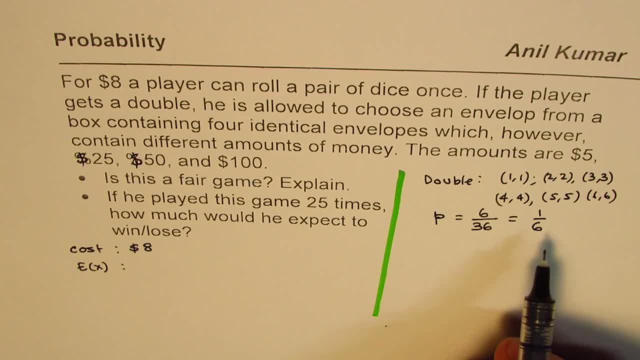 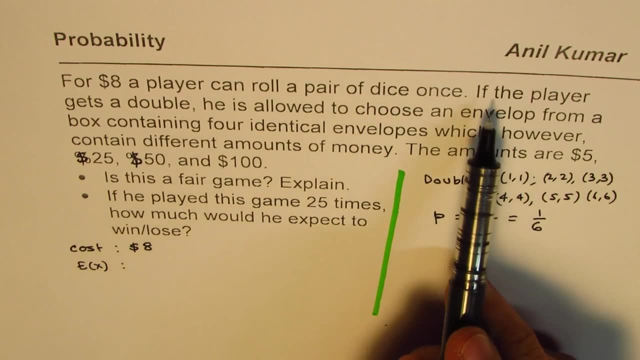 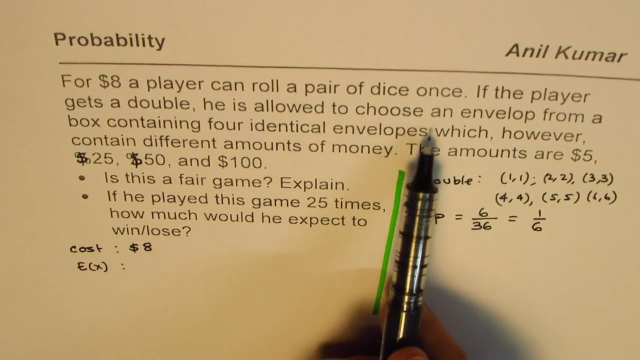 Now, if success is that, that is a success. Now let's look into this question. For $8,, a player can roll a pair of dice. If The player gets a double, if he gets a double, which probability is 1 out of 6, he is allowed to choose an envelope. 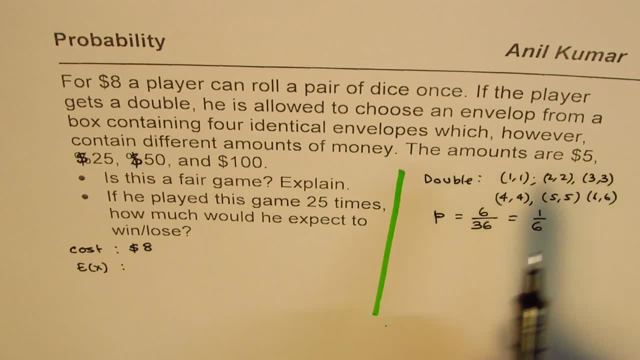 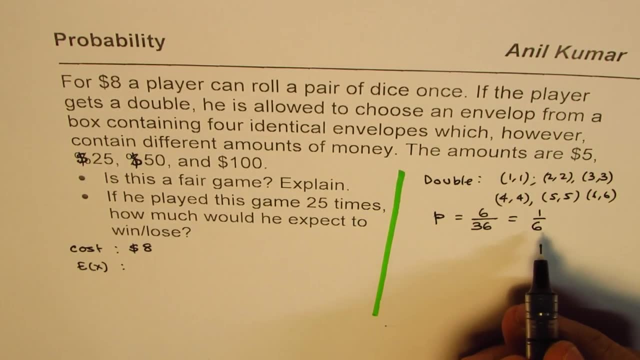 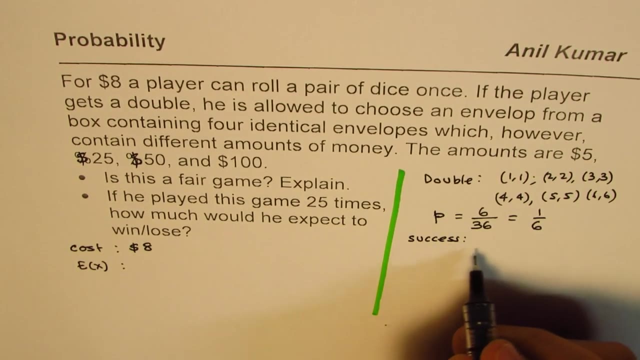 from a box containing four identical envelopes. So one event is followed by the other, and with an and condition. So the probabilities get multiplied, right. So for a success here, let's see success, right, So success here is 1 out of 6.. In that case, 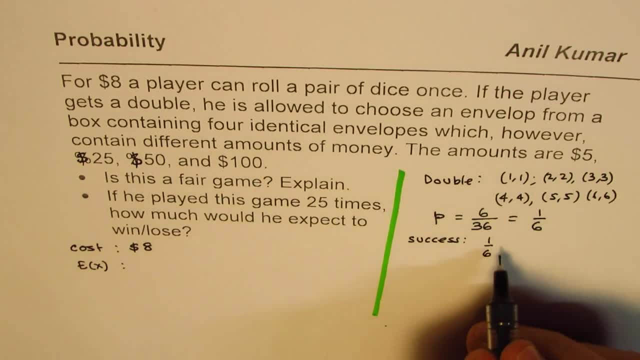 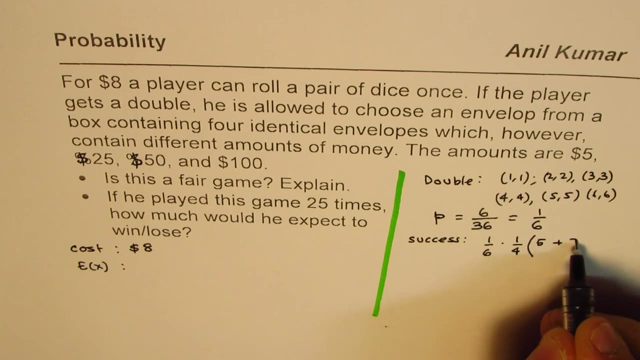 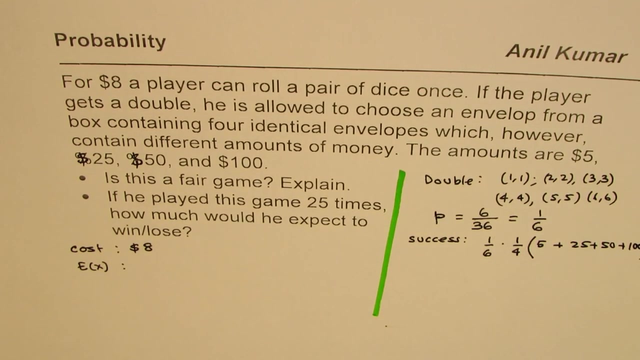 box containing four identical envelopes. So one-fourth is picking up, because there are four different envelopes, So one-fourth is picking up one of those. right, Which one of those? They have different amounts, So the amounts are 5, we're just adding them up: 25 plus 50 plus 100.. Is that okay? Does it make sense? So that is all. 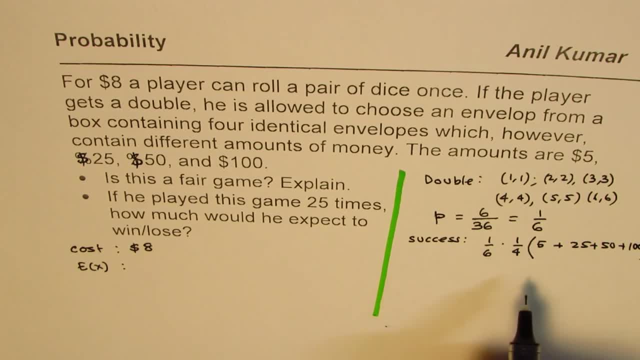 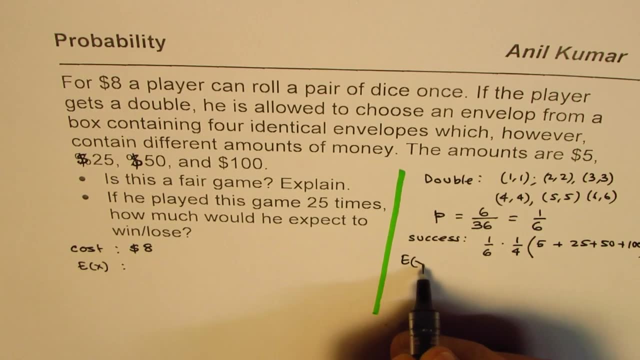 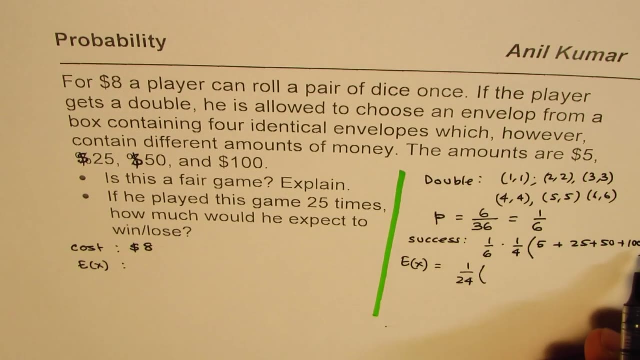 So if that is what is expected to win in a trial, do you understand? So that is your expected value. So let's calculate this. This is 1 over 24 of add all this, So so 150, 175, 180.. Is that okay? 180. 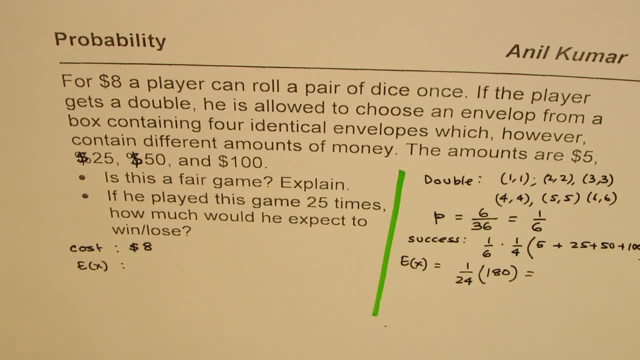 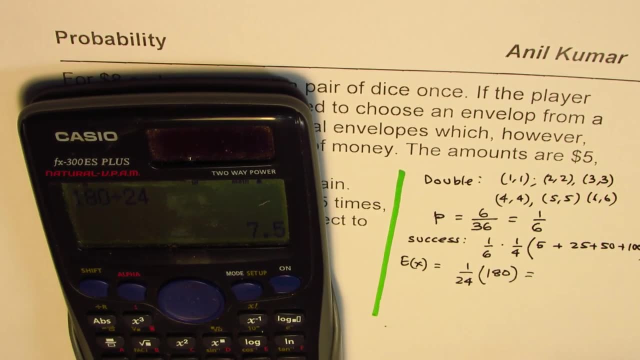 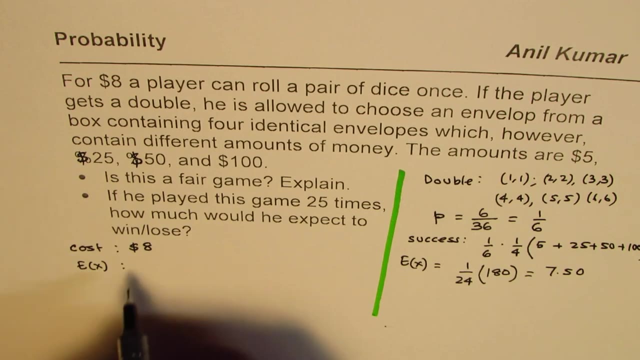 So we can always use calculator find this value: It is 180 divided by 24,, which is half of 15, or 750.. Okay, let me write 750.. So the expected value here in dollars is $7.50.. You are spending $8.. That means what? 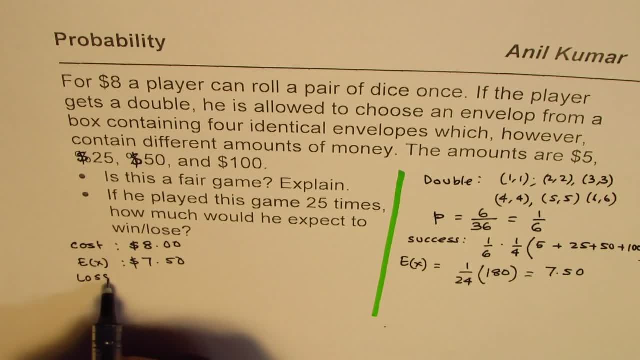 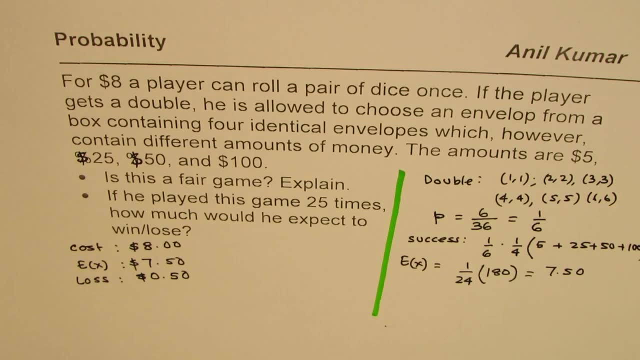 That means a loss of 50 cents. or say, do you see? So that is a loss of 50 cents. So should you call this a fair game, right? So we'll say not fair, So that is a loss of 50 cents. So should you call this a fair game, right? So we'll say not fair. 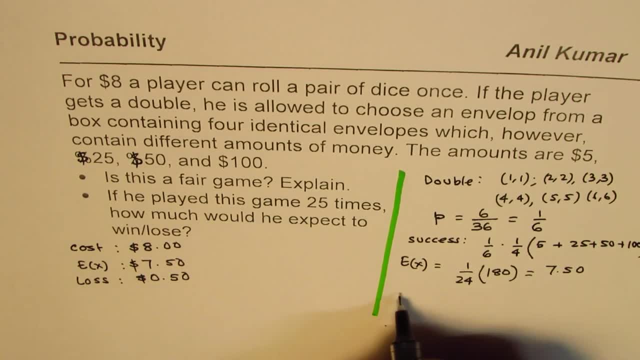 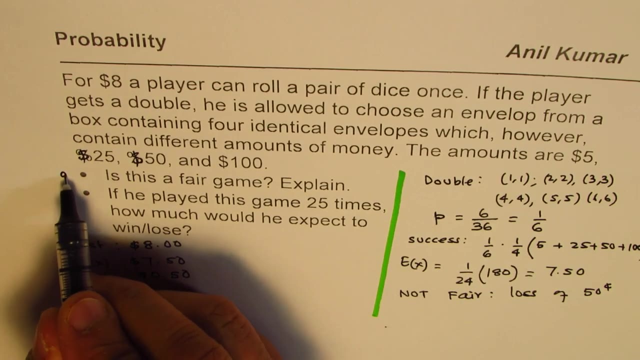 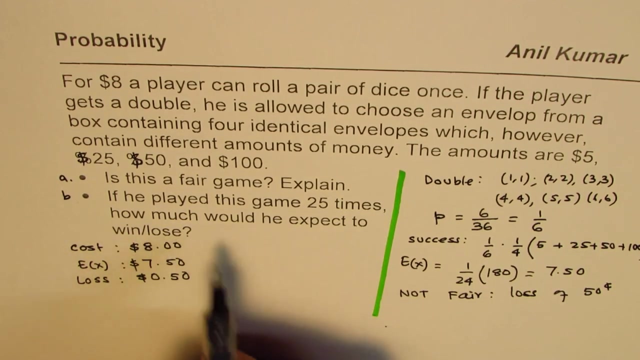 So should you call this a fair game, right? So we'll say not fair, As it gives a loss of 50 cents. Okay, That's one. Part B is: if a player, if he played this game 25 times, how much would he expect to lose? So so the part B answer is: expected loss.